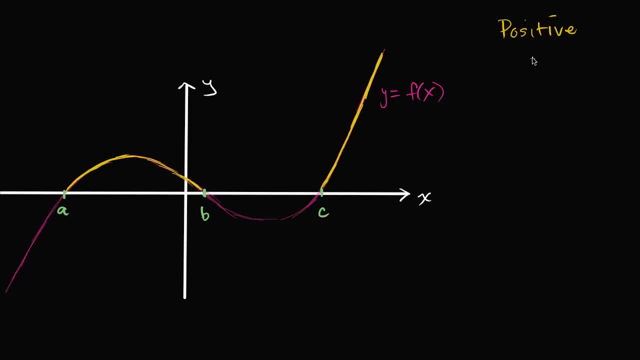 the value of our function is zero, but it's positive when x is between a and b, a and b, or if x is greater than c, X is. we could write it there: c is less than x, or we could write that x is. 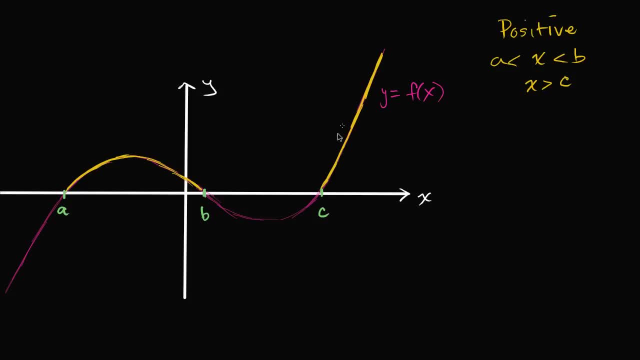 is greater than c. These are the intervals when our function is positive. Let me write this: f of x, f of x positive when x is in this interval or this interval or that interval. So when is f of x negative? 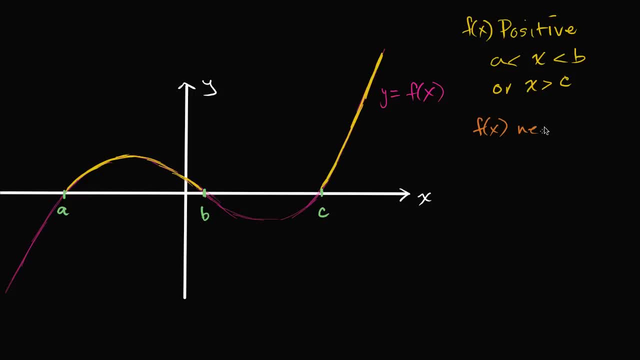 Let me do this in another color. F of x is going to be negative. Well, it's gonna be negative if x is less than a. so this is: if x is less than a, or if x is between b and c, then we see that f of x is below the x-axis. 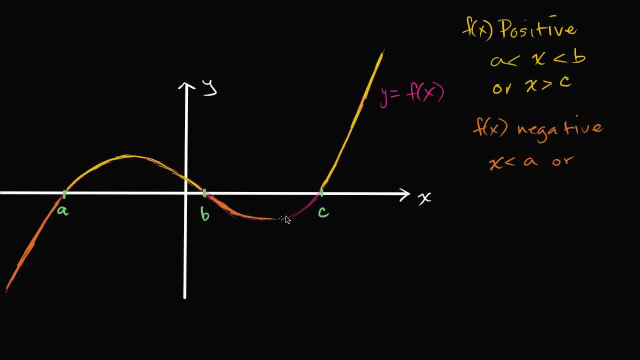 F of x is down here, so this is where it's negative. So here, or or x is between b or c. B x is between b and c, and I'm not saying less than or equal to, because if at b or c the value of the function, 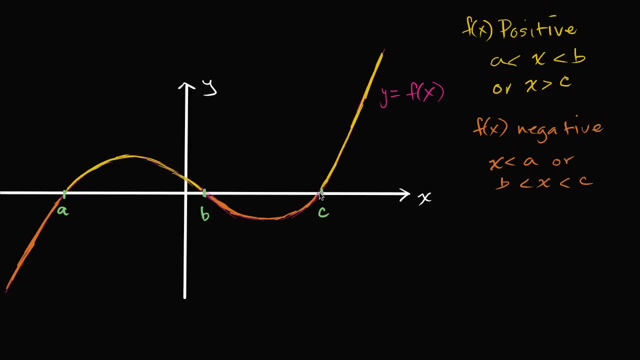 f of b is zero, f of c is zero. that's where we are actually intersecting the x-axis. So that was reasonably straightforward. Now let's ask ourselves a different question: When is the function increasing or decreasing? So when is f of x, f of x in increasing? 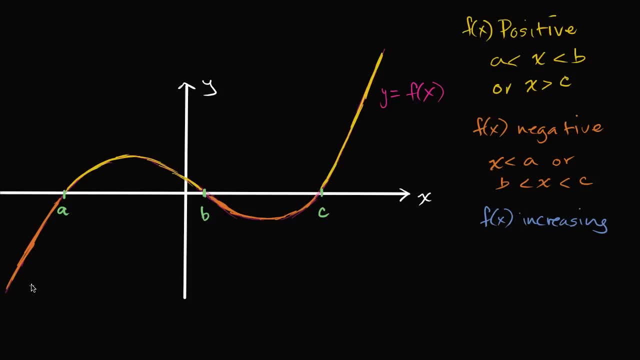 Well, increasing. one way to think about it is for every time that x is increasing, then y should be increasing. Or another way to think about it: you have a positive rate of change of y with respect to x. Or you could even think about it as: 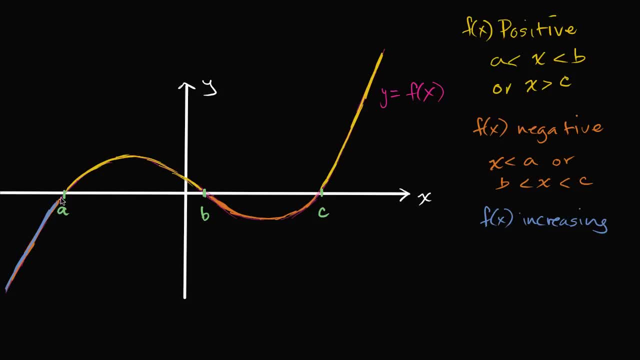 imagine if you had a tangent line at any of these points. if you had a tangent line at any of these points, the slope of that tangent line is going to be is going to be positive. But the easiest way for me to think about it is: 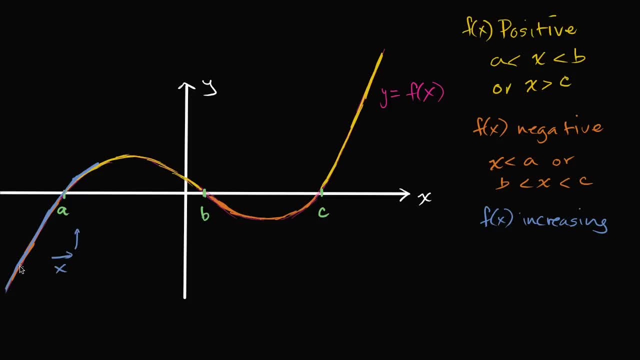 as you increase x, you're going to be increasing y. So where is the function increasing? Well, I'm doing it in blue, So it's increasing. right until we get to this, this point right over here, Right until we get to that point over there. 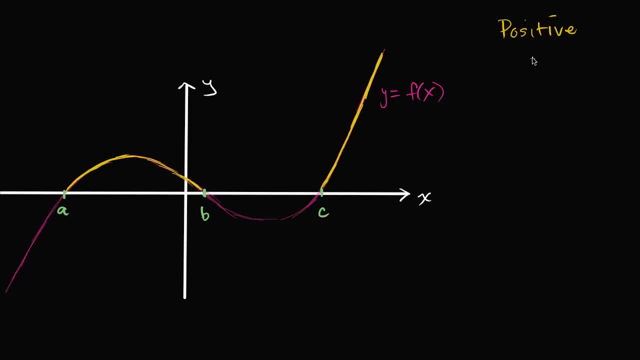 the value of our function is zero, but it's positive when x is between a and b, a and b, or if x is greater than c, X is. we could write it there: c is less than x, or we could write that x is. 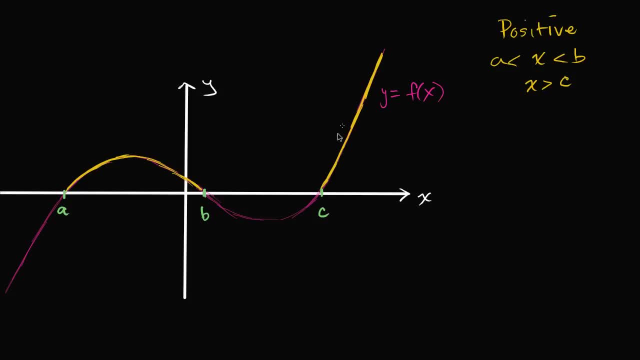 is greater than c. These are the intervals when our function is positive. Let me write this: f of x, f of x positive when x is in this interval or this interval or that interval. So when is f of x negative? 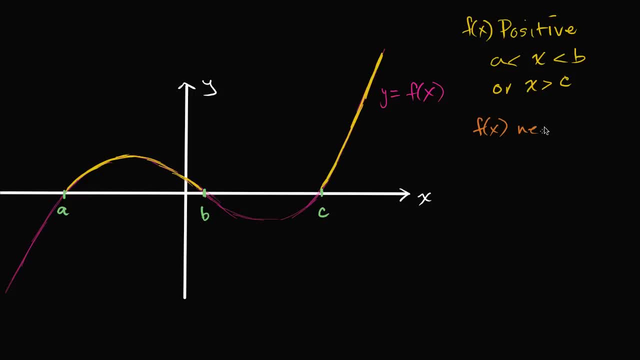 Let me do this in another color. F of x is going to be negative. Well, it's gonna be negative if x is less than a. so this is: if x is less than a, or if x is between b and c, then we see that f of x is below the x-axis. 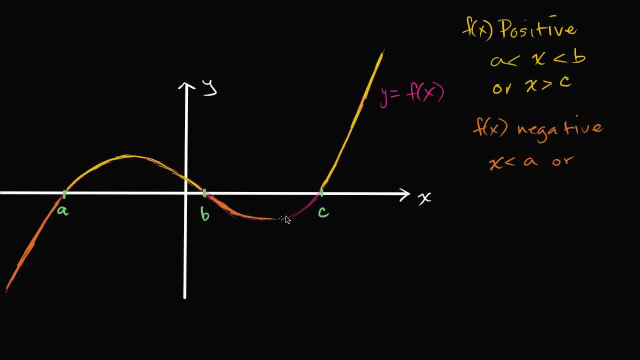 F of x is down here, so this is where it's negative. So here, or or x is between b or c. B x is between b and c, and I'm not saying less than or equal to, because if at b or c the value of the function, 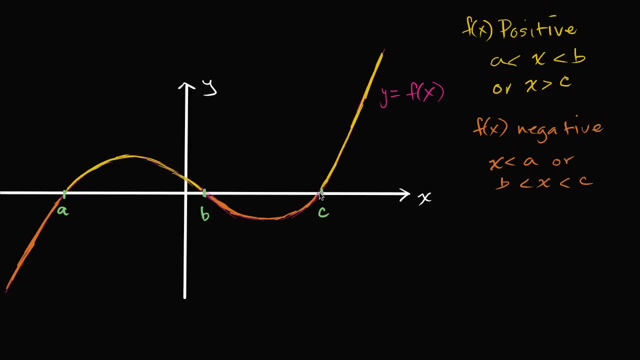 f of b is zero, f of c is zero. that's where we are actually intersecting the x-axis. So that was reasonably straightforward. Now let's ask ourselves a different question: When is the function increasing or decreasing? So when is f of x, f of x in increasing? 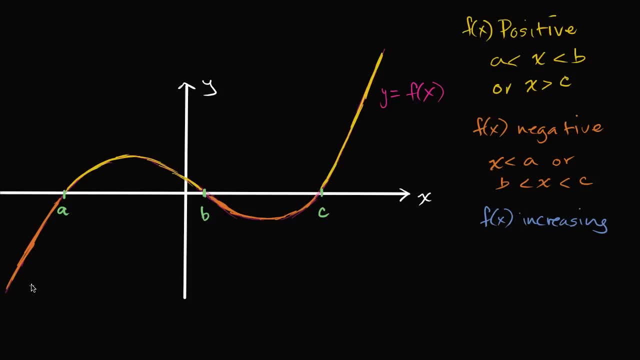 Well, increasing. one way to think about it is for every time that x is increasing, then y should be increasing. Or another way to think about it: you have a positive rate of change of y with respect to x. Or you could even think about it as: 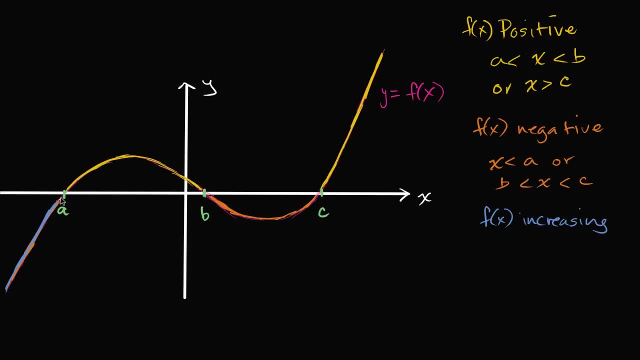 imagine if you had a tangent line at any of these points. if you had a tangent line at any of these points, the slope of that tangent line is going to be positive. But the easiest way for me to think about it is: as you increase x, you're going to be increasing y. 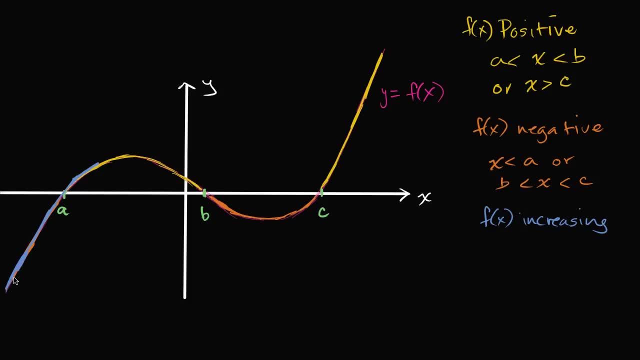 So where is the function increasing? Well, I'm doing it in blue. So it's increasing right until we get to this, this point right over here. Right until we get to that point over there, Then it starts decreasing until we get to this point. 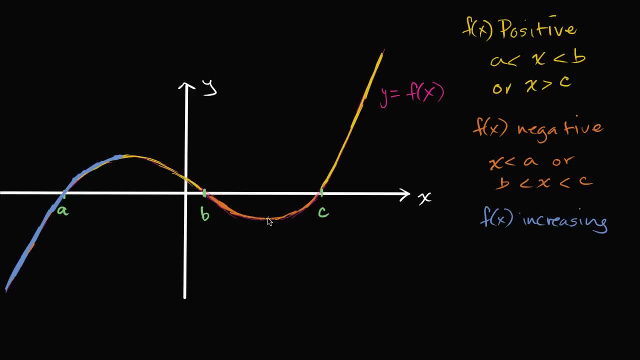 And then it starts decreasing until we get to this point right over here, and then it starts increasing again. It starts, it starts increasing again. So let me make some more, let me make some more labels here. So let's say that this, this is x equals d. 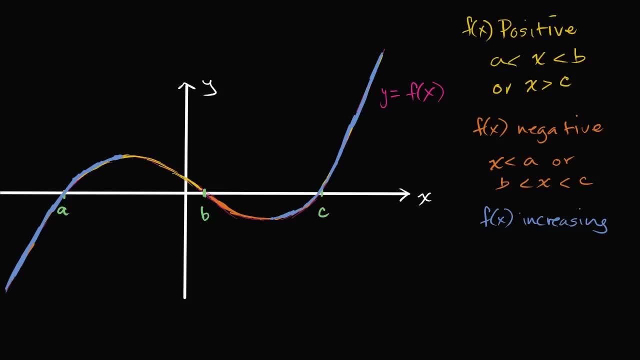 and that this right over here, actually let me do that green color. So let's say this is x equals d- now, it's not a d, b, But you get the picture. And let's say that this is x is equal to. 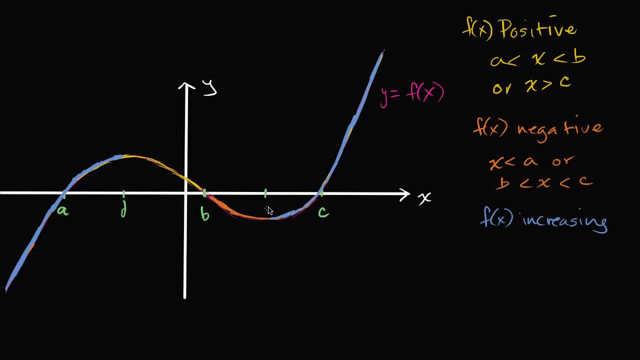 x is equal to. let me do it a little bit: x is equal to e, x is equal to e. So when is this function increasing? Well, it's increasing. if x is less than d, x is less than d, And I'm not going to say less than or equal to. 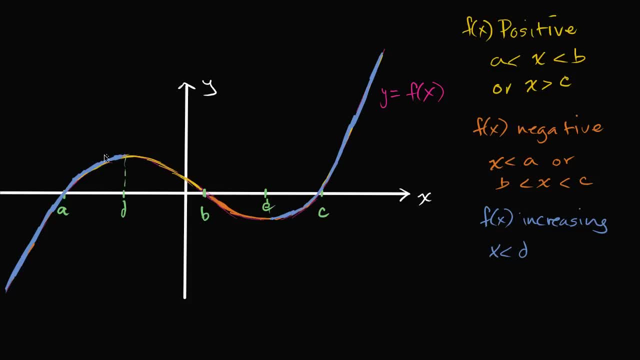 because right at x equals d, it looks like, just for that moment, the slope of the tangent line looks like it would be, it would be constant. So we're going from increasing to decreasing. So right at d, we're neither increasing or decreasing. 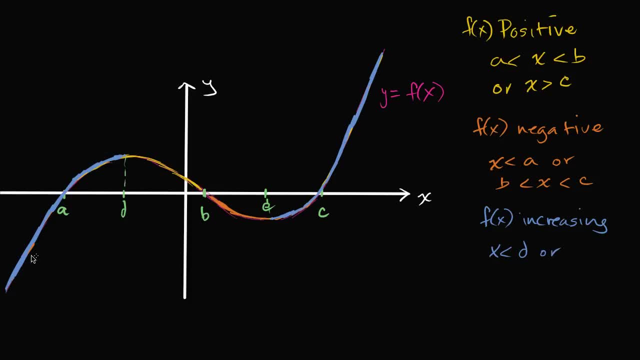 But then we're also increasing. So if x is less than d, or x is greater than e, Or x is greater than e, And where is f of x decreasing? So f of x. let me do this in a different color. 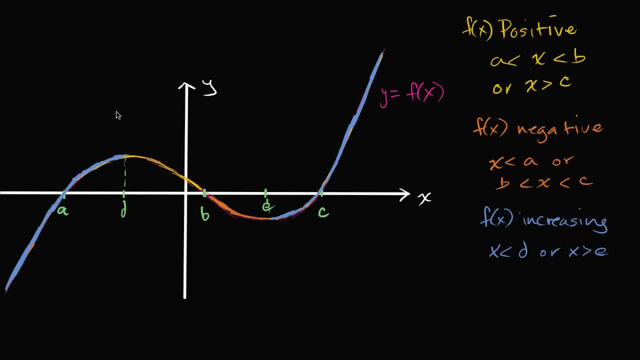 When is- let me pick a move- So f of x, decreasing, decreasing. Well, it's going to be right over here. It's going to be right between d and e, Between x equals d and x equals e, But not exactly at those points. 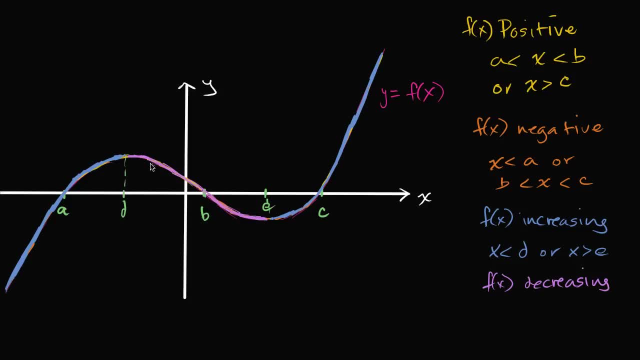 because at both of those points you're neither increasing nor decreasing. But you see, right over here, as x increases, as you increase your x, what's happening to your y? If you go from this point and you increase your x, what happened to your y? 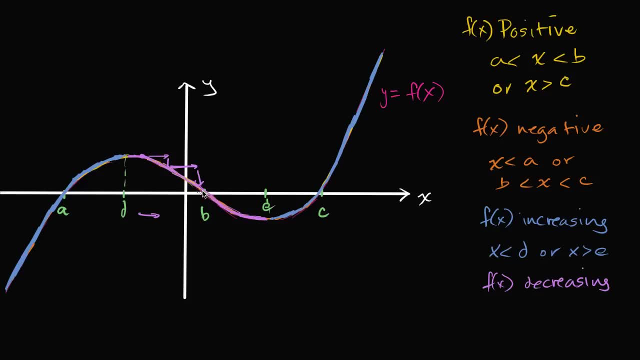 Your y has decreased. You increase your x. your y has decreased. You increase your x. y has decreased. Increase x. y has decreased All the way until this point over here. So f of x is decreasing for x between d and e. 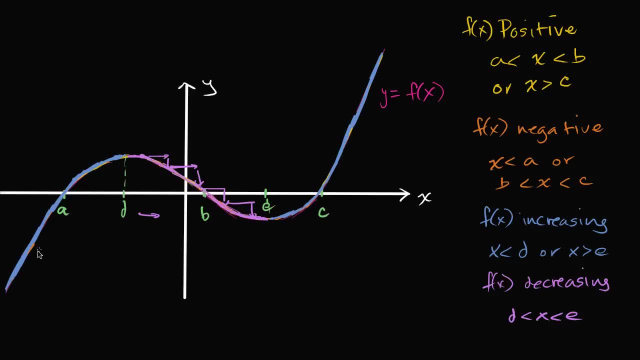 So hopefully that gives you a sense of things. Notice, these aren't the same intervals That we are. the intervals where we're positive or negative don't perfectly coincide with when we are increasing or decreasing, So it's very important to think about these separately. even though they kind of sound the same, All right. 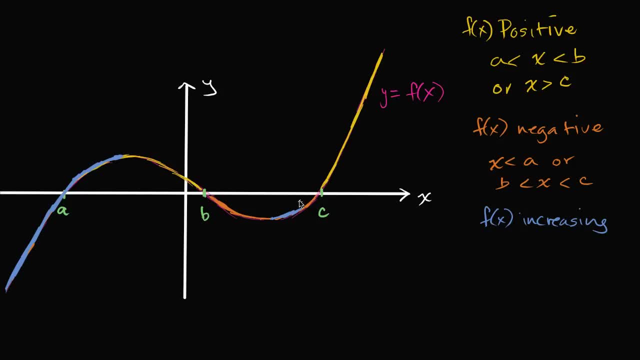 right over here, and then it starts increasing again. It starts, it starts increasing again. So let me make some more, let me make some more labels here. So let's say that this, this is x equals d and that this, right over here, 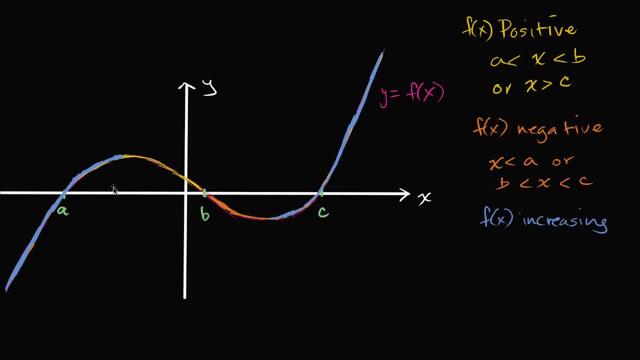 actually let me do that green color. So let's say this is x equals d. now it's not a d, b, But you get the picture. And let's say that this is x is equal to, x is equal to. let me do it a little bit. 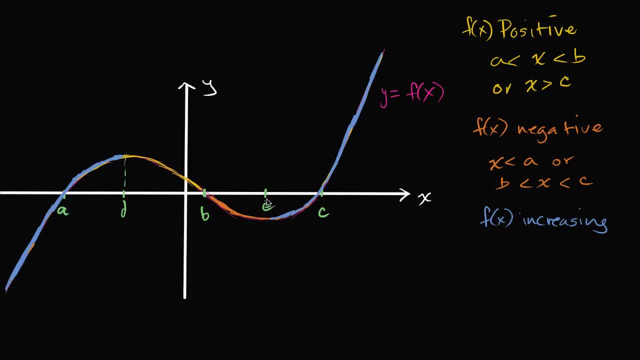 x is equal to e, x is equal to e. So when is this function increasing? Well, it's increasing. if x is less than d, x is less than d, And I'm not going to say less than or equal to, because right at x equals d, it looks like. 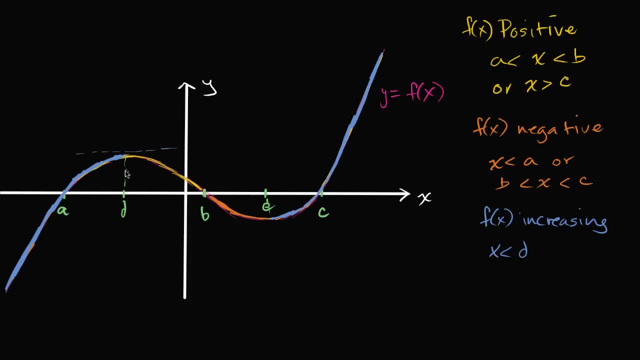 just for that moment, the slope of the tangent line looks like it would be. it would be constant. We're going from. we're going from increasing to decreasing. So, right at d, we're neither increasing or decreasing, But then we're also increasing. 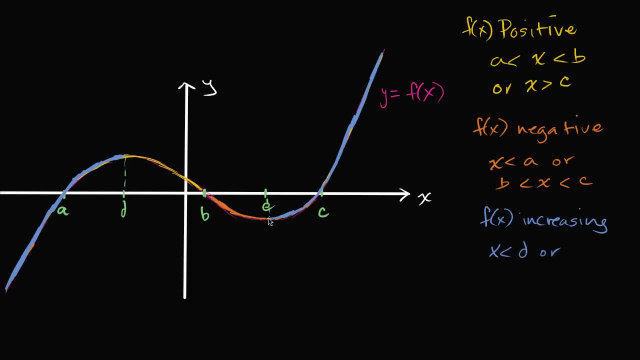 So if x is less than d, or x is greater than e, or x is greater than e, And where is f of x decreasing? So f of x, let me do this in a different color. When is? let me pick a move. 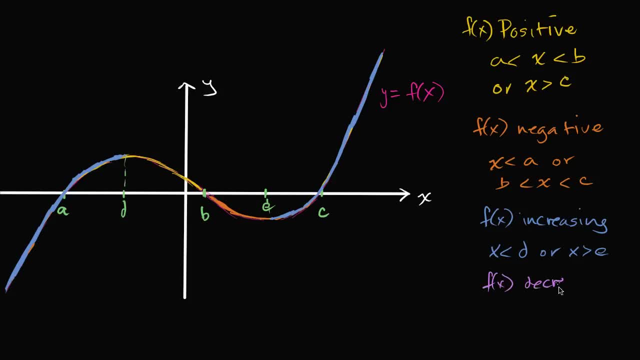 So f of x decreasing, decreasing. Well, it's going to be right over here, It's going to be right between d and e, between x equals d and x equals e, But not exactly at those points, because at both of those points, 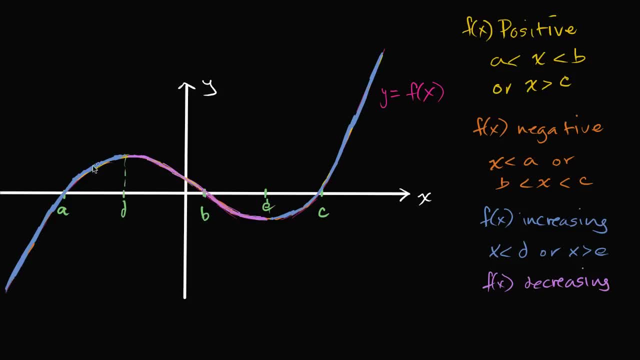 you're neither increasing nor decreasing. But you see, right over here, as x increases, as you increase your x, what's happening to your y? If you go from this point and you increase your x, what happened to your y? Your y has decreased. 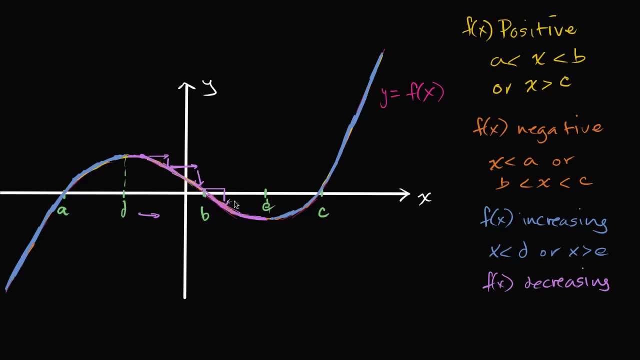 You increase your x, your y has decreased. You increase your x. y has decreased. Increase x. y has decreased all the way until this point over here. So f of x is decreasing for x between d and e. So hopefully that gives you a sense of things.